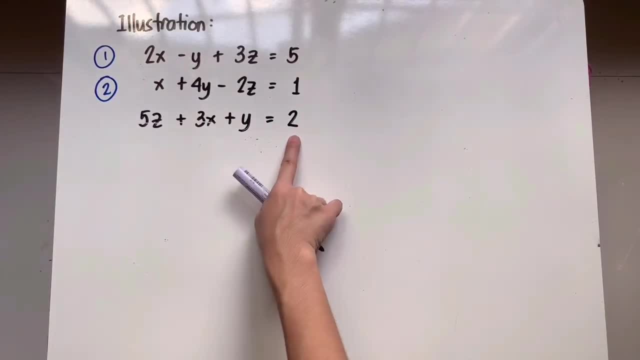 And it is noticeable that the third equation is not arranged in such manner. So for the third equation, that would be 3x plus y plus 5z and that's equivalent to 2.. So these three equations will be the equations we'll be solving using matrix inversion. 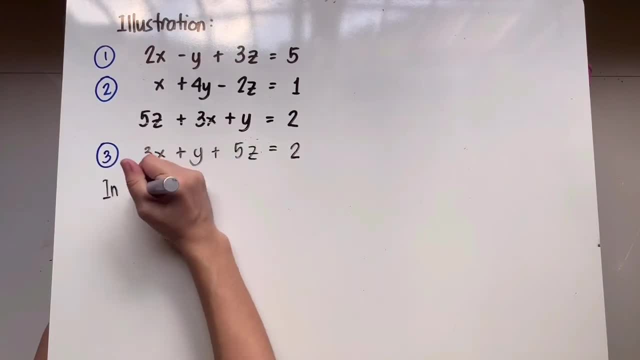 But before that let's write this in matrix form again. So in matrix form, let's start with our coefficient matrix first, And we'll have to write down the coefficients of each equation in the order x, y, z again. So that would be 2, negative 1, 3.. 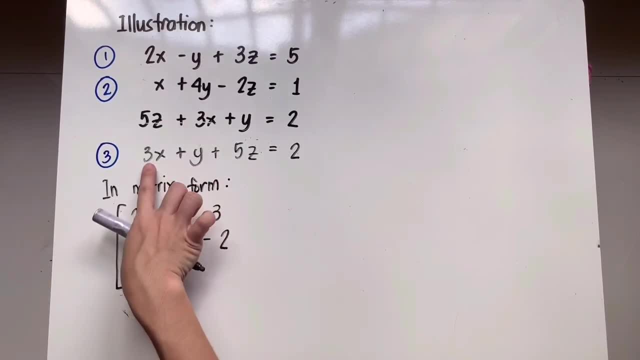 We have 1,, 4, and negative 2.. And for the third equation we'll follow this one, because this is arranged in x, y, z, And that would be 3,, 1, and 5. That will be multiplied to a column vector of the variables x, y and z. 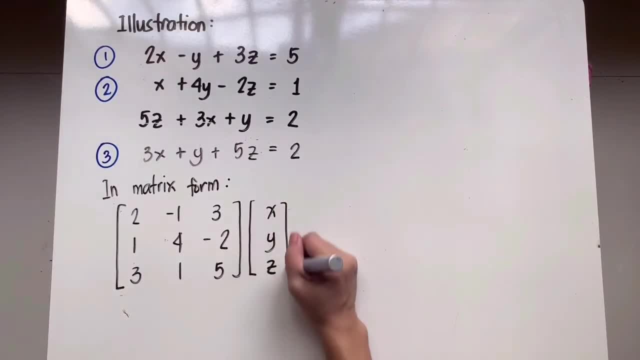 x, y, z, And that would be equivalent to the constants in our equations, And that would be 5,, 1, and 2.. Matrix inversion solution follows division of matrices, And that is, if you want to solve for x, y, z, you have to divide both sides by this matrix. 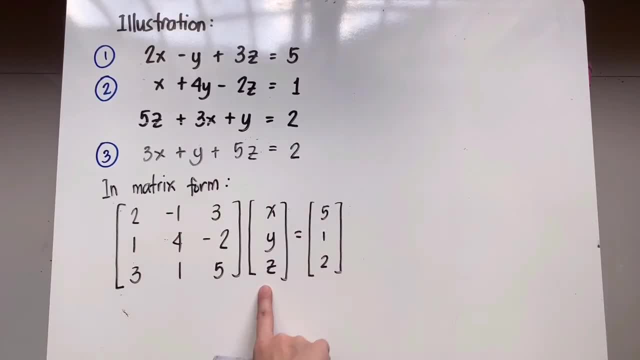 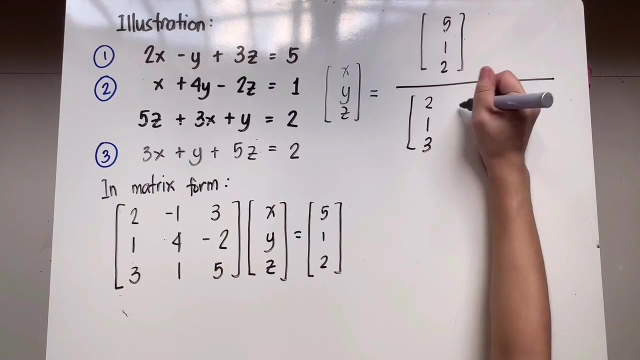 So what will happen here is that you'll be left with the variable matrix Variables on the left side, that would be x, y and z will be equivalent to this, the right side, which is 5, 1, and 2, to be divided by the coefficient matrix, which is 2, 1, 3, negative 1, 4, 1, and 3, negative 2, 5.. 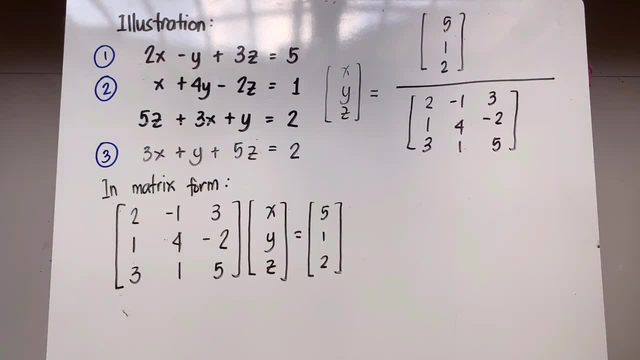 For this we're going to use principles of division, The division of matrices wherein the denominator becomes a multiplicand by taking its inverse. So the solution here is that x, y, z matrix will be equivalent to this matrix, your coefficient, So 2, 1, 3, negative, 1, 4, 1, 3, negative, 2, 5.. 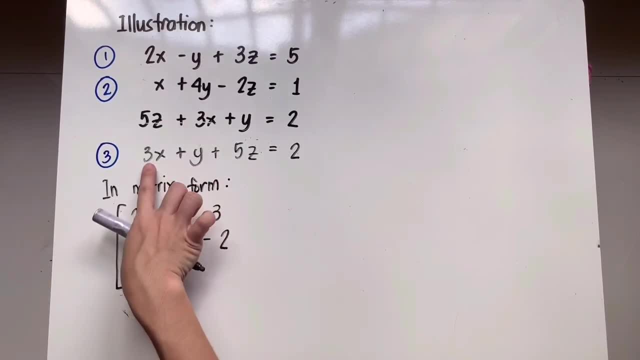 We have 1,, 4, and negative 2.. And for the third equation we'll follow this one, because this is arranged in x, y, z, And that would be 3,, 1, and 5. That will be multiplied to a column vector of the variables x, y and z. 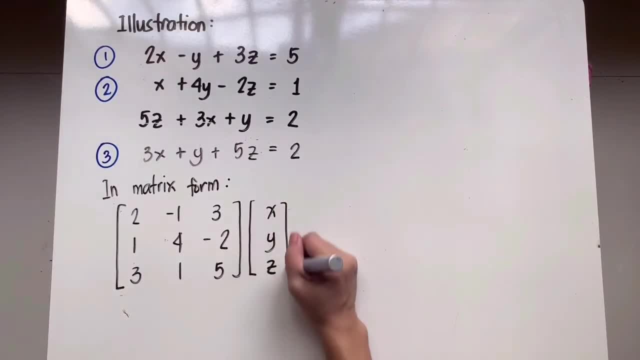 x, y, z, And that would be equivalent to the constants in our equations, And that would be 5,, 1, and 2.. Matrix inversion solution follows division of matrices, And that is, if you want to solve for x, y, z, you have to divide both sides by this matrix. 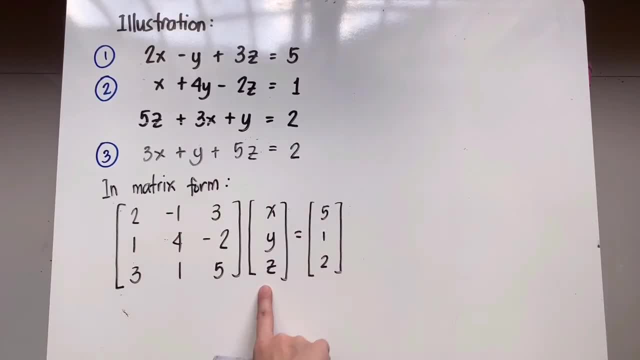 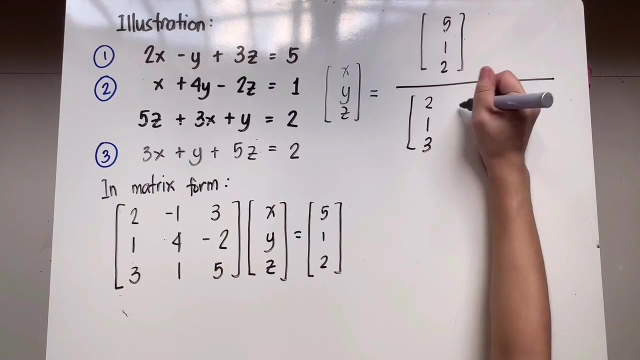 So what will happen here is that you'll be left with the variable matrix Variables on the left side, that would be x, y and z will be equivalent to this, the right side, which is 5, 1, and 2, to be divided by the coefficient matrix, which is 2, 1, 3, negative 1, 4, 1, and 3, negative 2, 5.. 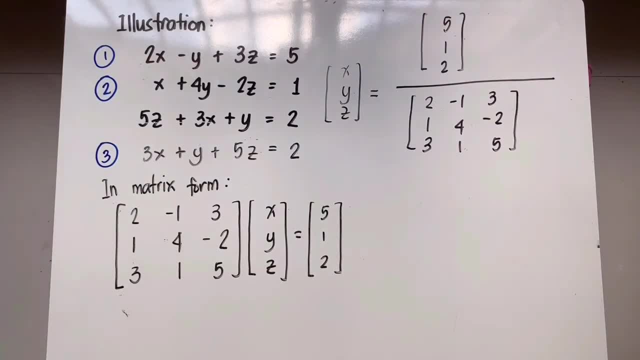 For this we're going to use principles of division, The division of matrices wherein the denominator becomes a multiplicand by taking its inverse. So the solution we're going to use here is that x, y, z matrix will be equivalent to this matrix, your coefficient. 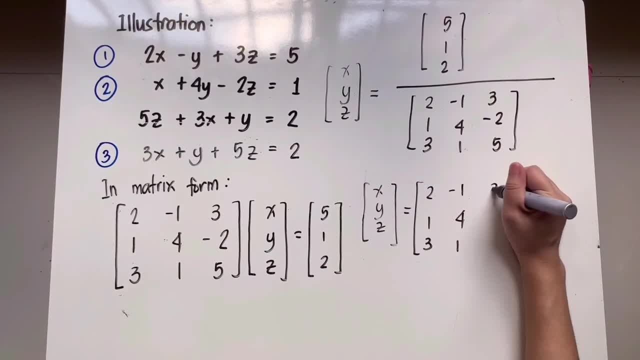 So 2, 1, 3, negative 1, 4, 1, 3, negative 2, 5.. Inverse of that To be multiplied, To be multiplied to your numerator, which is 5, 1, 2.. 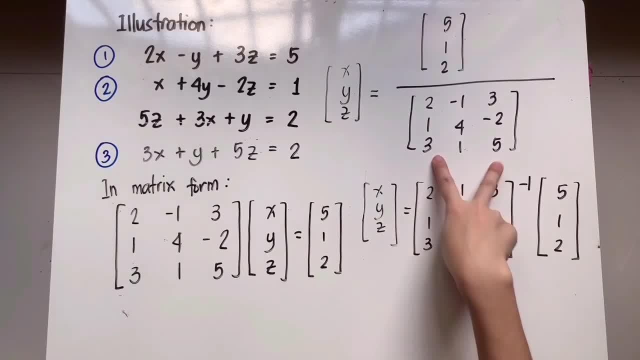 Okay, again, your denominator becomes a multiplicand in the numerator and not a multiplier. The sequence cannot be reversed because multiplication is not commutative. So for that we're going to take the inverse of this matrix first. Okay, Continuing our matrix inversion solution. 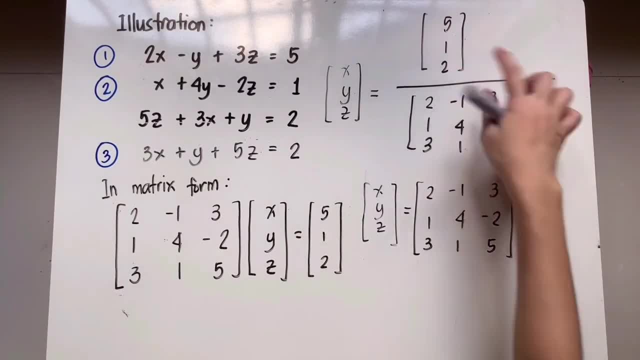 Inverse of that to be multiplied To your numerator, which is 5, 1, 2.. Okay, again, your denominator becomes a multiplicand in the numerator and not a multiplier. The sequence cannot be reversed because multiplication is not commutative. 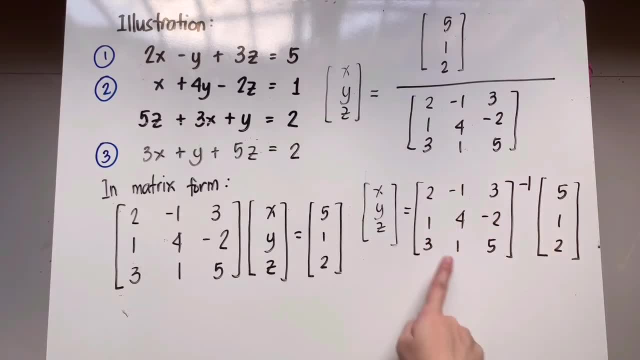 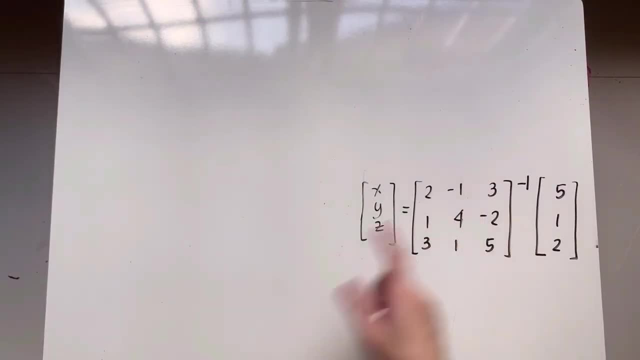 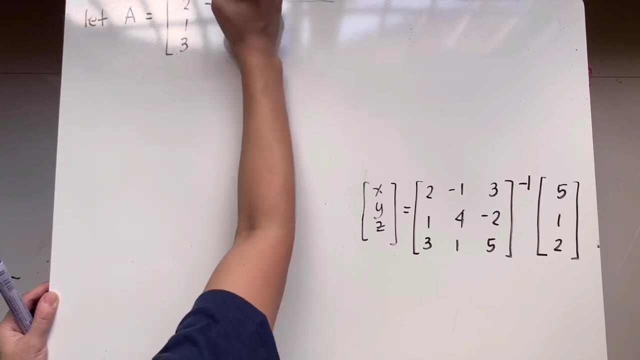 So for that we're going to take the inverse of this matrix first. Okay, continuing our matrix inversion solution. So let's say our coefficient matrix, Let's let that As matrix A, and that is your 2, 1, 3, negative, 1, 4, 1, 3, negative, 2, 5.. 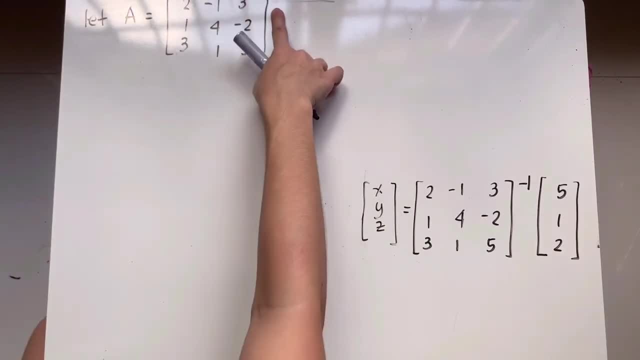 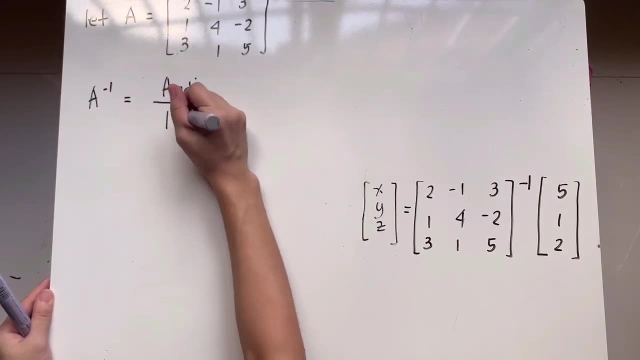 To take A inverse or to take the inverse of the coefficient matrix. the solution for A inverse is simply A adjoint divided by the determinant of A, And we know for sure that the determinant of A is not 0 because we've solved this in the previous solution that we've had. 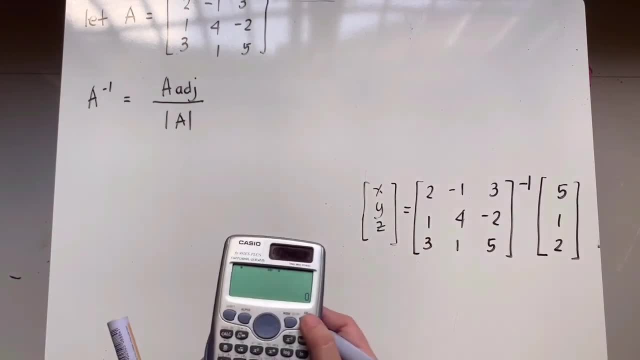 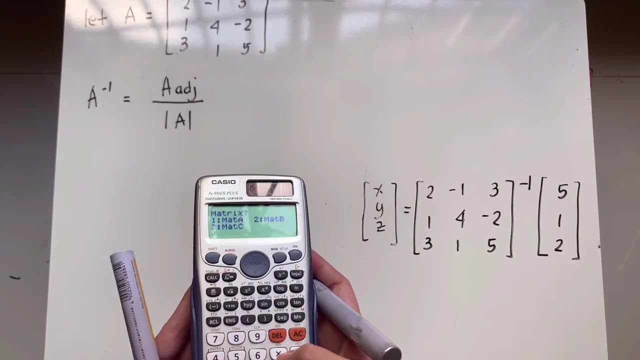 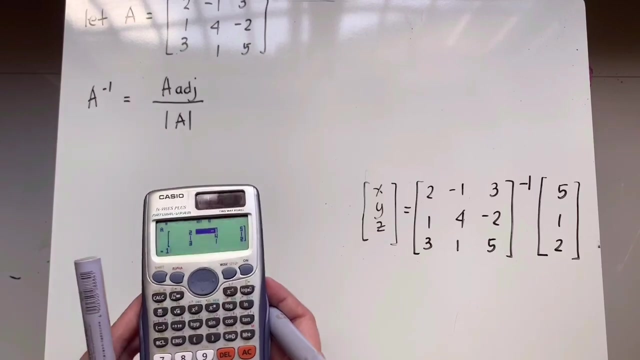 Okay, Okay, And to show you again, I'm going to take my calculator here to show you that shift matrix, data matrix A, and input this coefficients or entries to our calculator. You have 2, negative 1, 3, 1, 4, negative 2, and 3, 1, 5.. 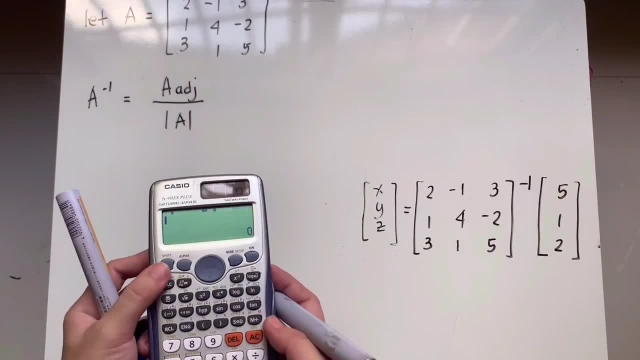 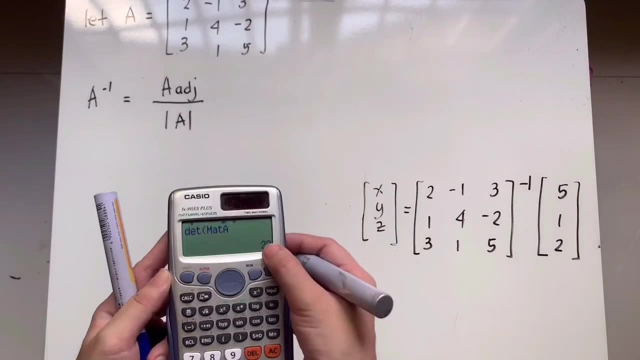 And it will show you that We'll clear the screen. Shift matrix determinant 7.. Shift The matrix, the matrix, the determinant of matrix A, and that gives us 22.. So the determinant of A gives us 22,, which means we have an inverse. 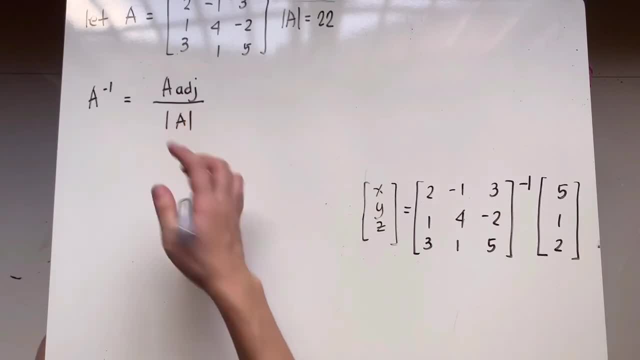 So if we've solved, if we have solved for the determinant, we can proceed in taking the adjoint of matrix A And for that adjoint, if you can still remember, we are going to replace, We are going to replace every entries of their minors. 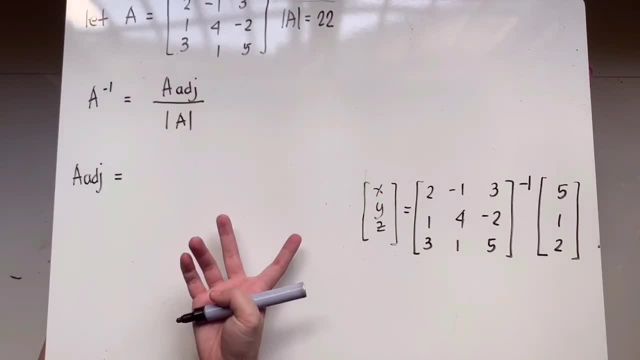 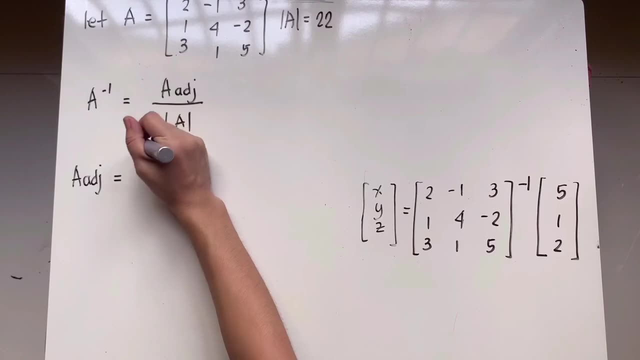 Place sign so that they become cofactors and then take its transpose. That will give you your adjoint matrix, Therefore, okay, we're going to cross out 2.. The remaining elements would be this one. So we're going to take the determinant of that to represent its minor. 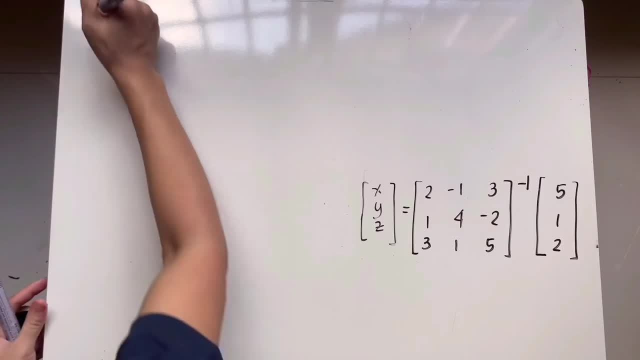 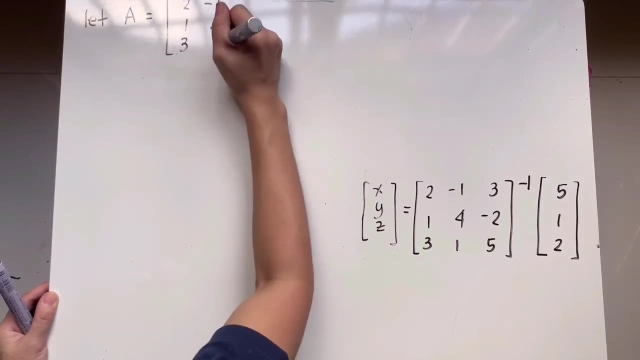 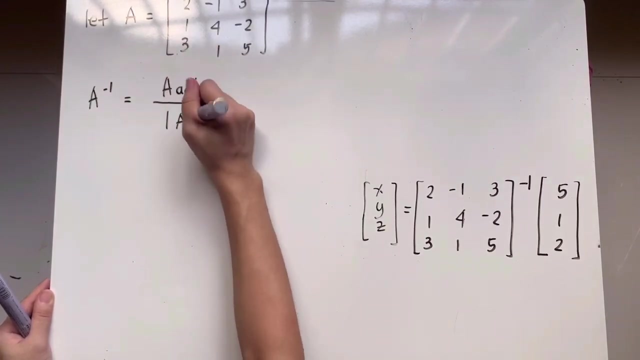 So let's say our coefficient matrix, Let's let that As matrix A, and that is your 2, 1, 3, negative 1, 4, 1, 3, negative 2, 5. To take A inverse, or to take the inverse of the coefficient matrix, the solution for A inverse is simply A adjoint divided by the determinant of A. 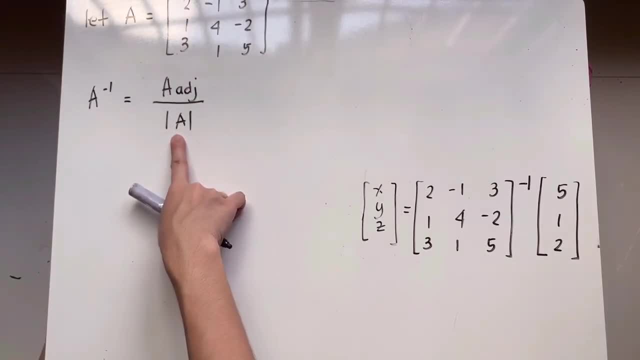 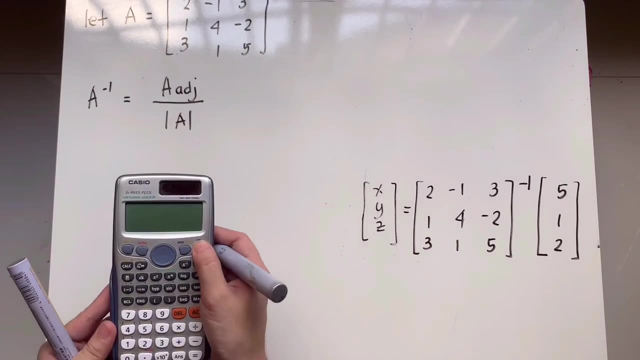 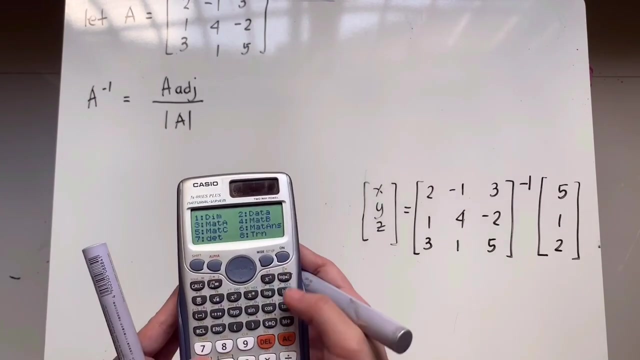 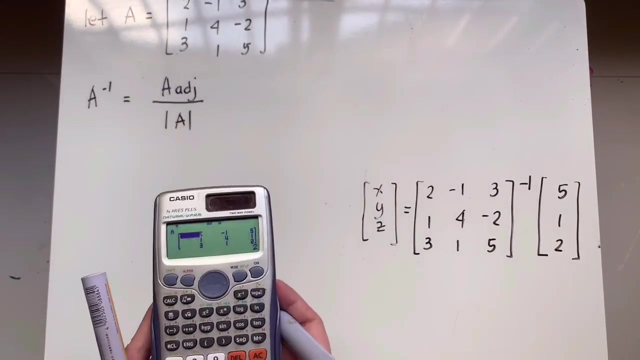 And we know for sure that the determinant of A is not 0 because we've solved this in the previous solution that we've had. Okay, And to show you again, I'm going to take my calculator here to show you that shift matrix, data, matrix A, and input this coefficients or entries to our calculator. 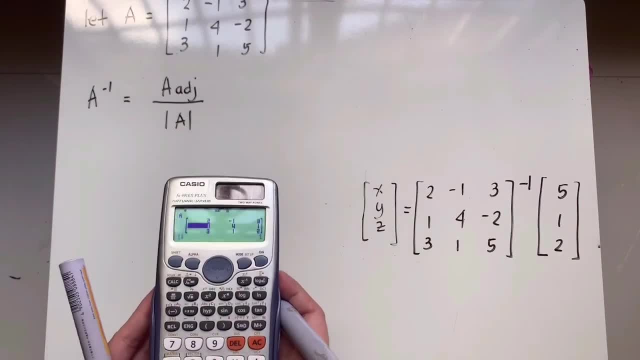 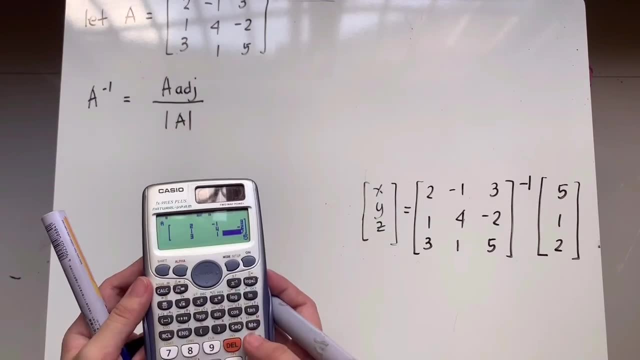 You have 2, negative 1, 3, 1, 4, negative 2, and 3, 1, 5.. And it will show you that We'll clear the screen: Shift matrix determinant 7.. 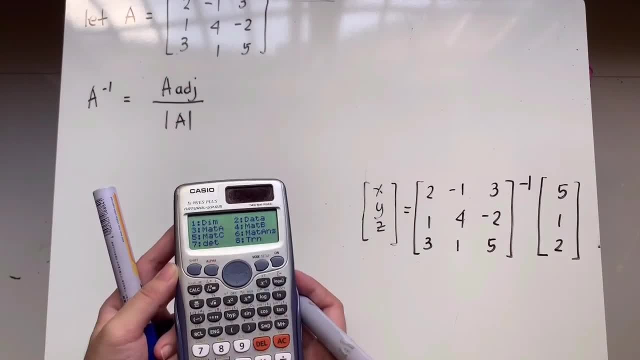 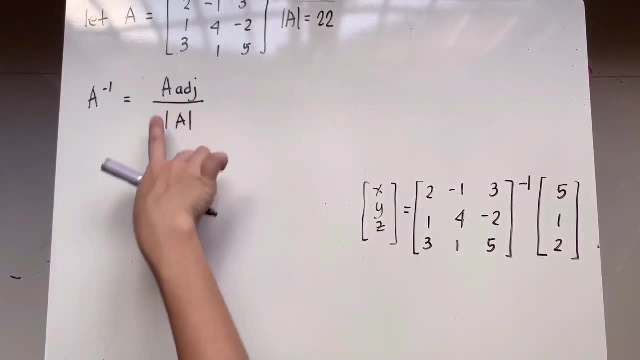 Shift matrix, the determinant of matrix A, and that gives us 22.. So the determinant of A gives us 22, which means we have an inverse. So if we have solved for the determinant, we can proceed in taking the adjoint of matrix A. 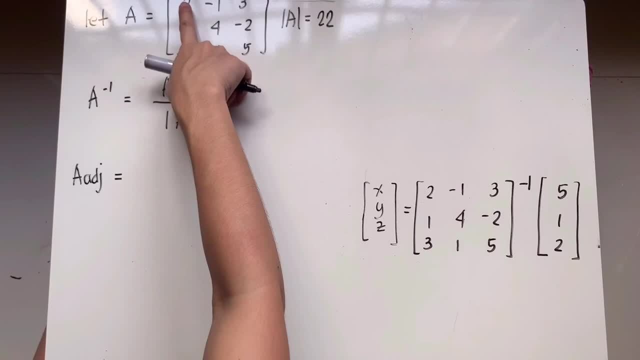 And for that adjoint, if you can still remember, we are going to replace, We're going to replace, We're going to replace each entries of their minors Place sign so that they become cofactors, and then take its transpose. That will give you your adjoint matrix. 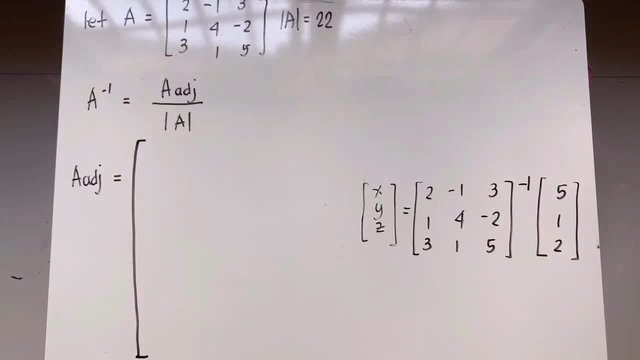 Therefore, we're going to cross out 2.. The remaining elements would be this one, So we're going to take the determinant of that to represent its minor, That's 4, 1, negative 2, and 5.. Next, remove this element. 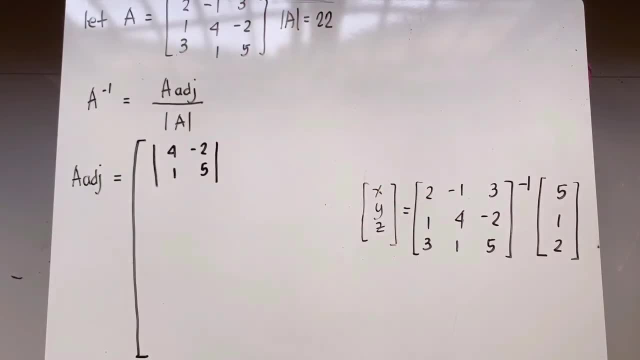 Cross this out, You'll be left with this: 4 entries, And that gives us 1, 3, negative 2, 5.. Next, cross this out. You'll get this. So you'll take its determinant: 1, 3, 4, 1.. 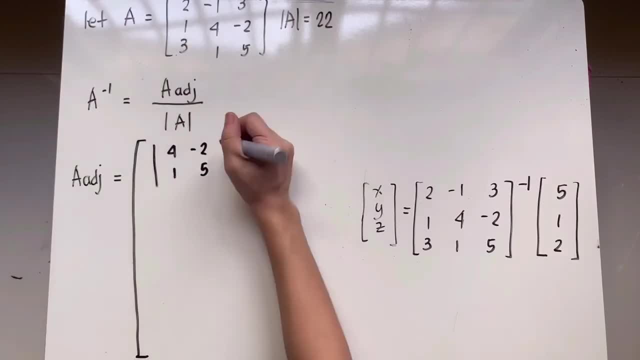 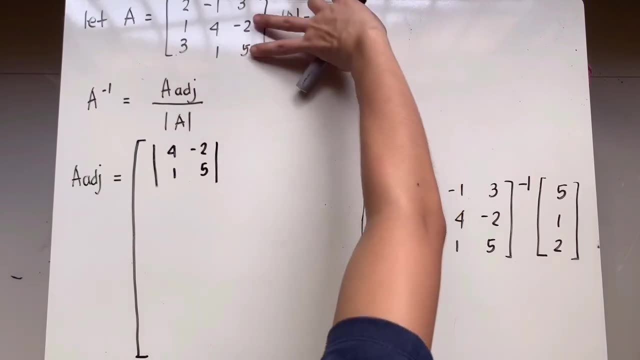 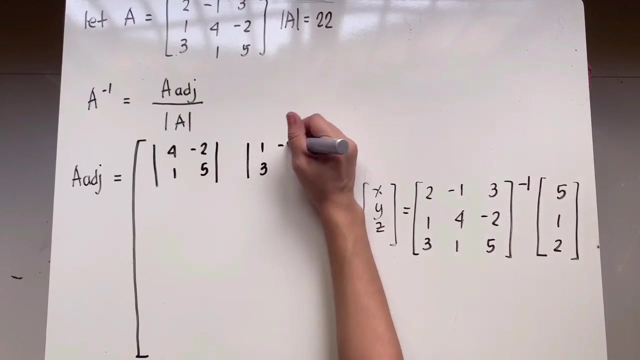 That's 4, 1, negative, 2, and 5.. Next, remove this element, Cross this out. You'll be left with this: 4 entries And that gives us 1, 3, negative 2, 5.. 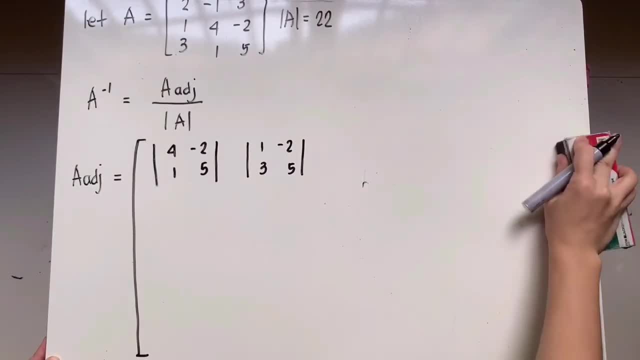 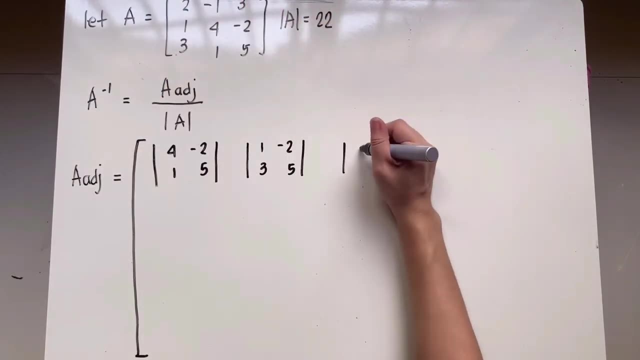 Next, Cross this out, You'll get this. So you'll take its determinant: 1,, 3,, 4,, 1.. And then we'll move to the second row. So cross this out, You'll get this. 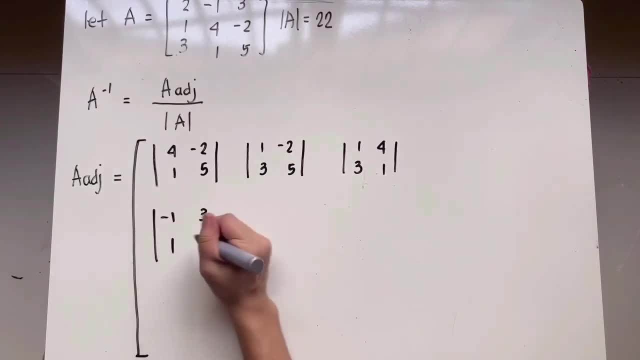 That gives us negative 1,, 3,, 1, 5.. Cross the middle element, You'll get all this: 4. And that would be the determinant of 2,, 3,, 3,, 5. And then for element 2,, 3.. 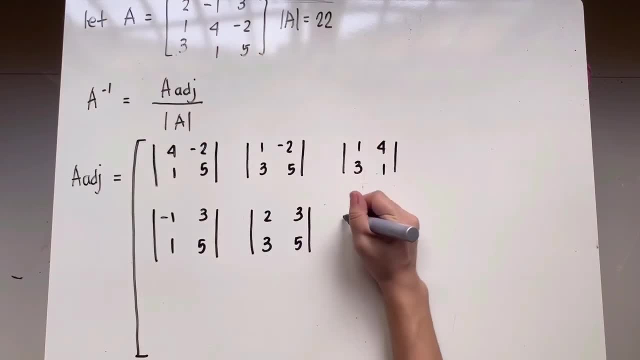 So cross element 2, 3.. You'll get this, So we'll take its determinant, That's 2, negative 1, 3, 1.. And then last row, So cross this out. You'll get this 4.. 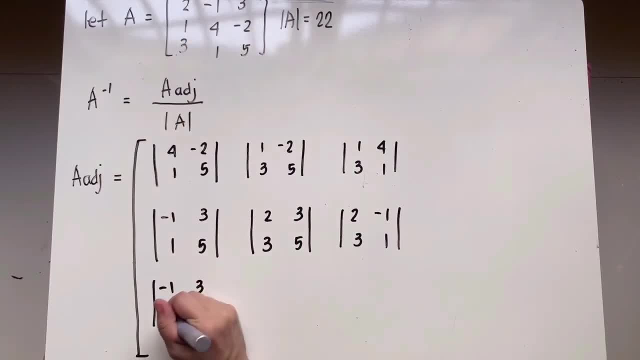 Determinant of that is negative 1, 3.. 4, negative 2.. Cross this out. You'll get 2, 1, 3, negative 2. And then cross this element out. That would be our last determinant. 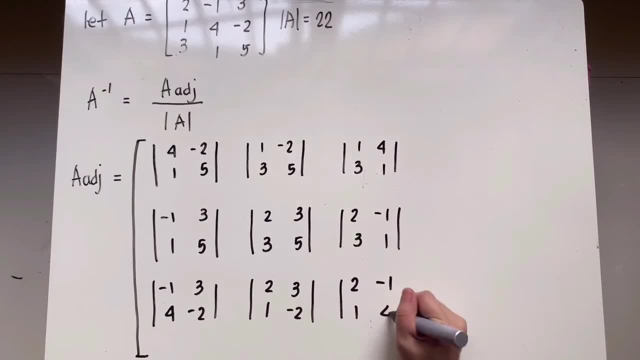 So, crossing this out, you'll get 2, negative 1, 1, 4.. Remember that We have to take. We have to replace Every element or entry by their cofactor, And the ones we took are just minors. 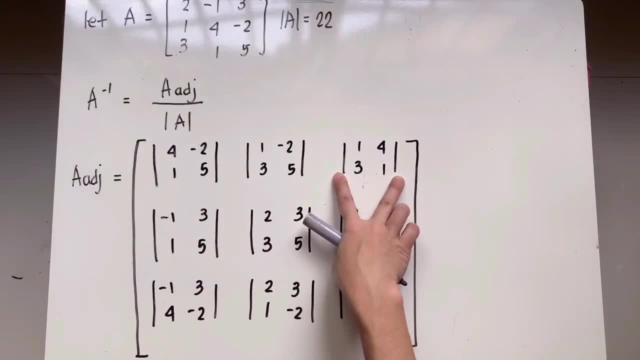 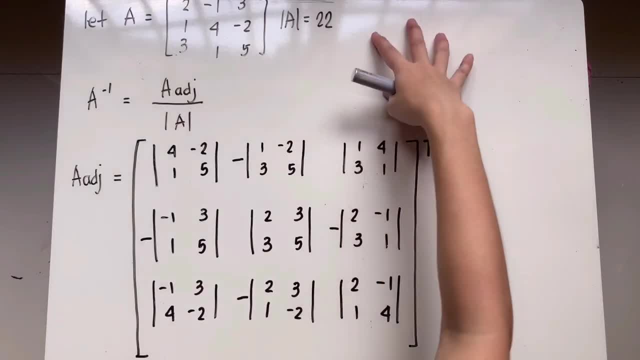 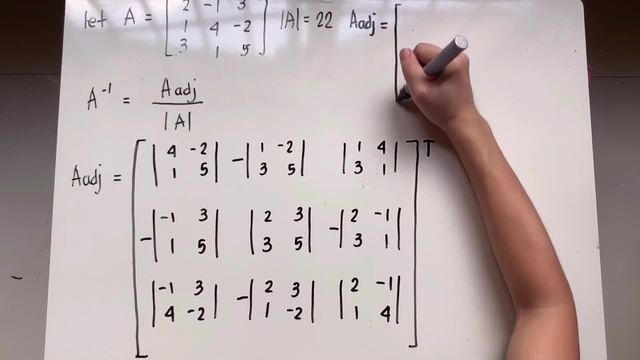 And that gives you your adjoint matrix. So let's continue that over here. I think this fits here. So for A adjoint That would be equivalent to: So we have 20 minus 20 minus negative 2.. 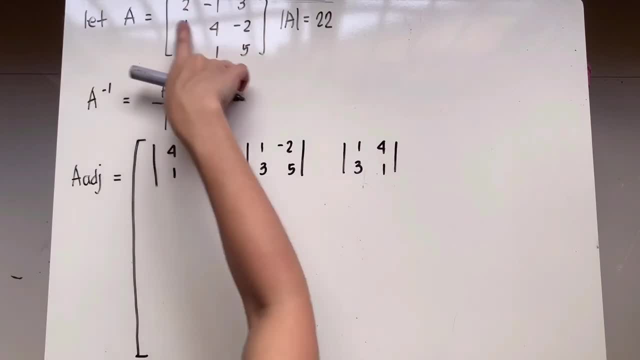 And then we'll move to the second row. So cross this out, You'll get this. That gives us negative 1, 3, 1, 5.. Cross the middle element, You'll get all this: 4.. And that would be the determinant of 2, 3, 3, 5.. 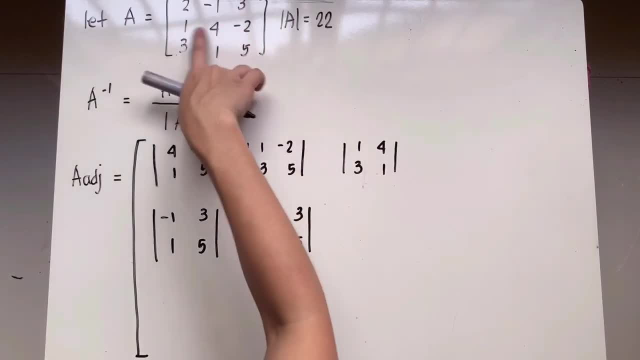 And then for element 2, 3.. So cross element 2, 3.. You'll get this, So we'll take its determinant, That's 2, negative 1.. 3, 1.. And then last row: 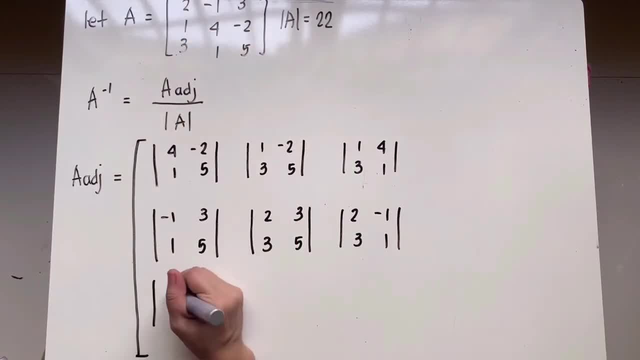 Cross this out, You'll get this: 4. Determinant of that is negative 1, 3.. 4, negative 2.. Cross this out, You'll get 2, 1.. 3, negative 2. And then cross this element out. 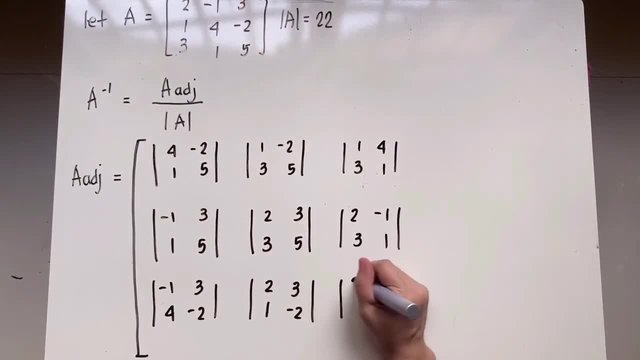 That would be our last determinant. So, crossing this out, you'll get 2, negative 1.. 1, 4.. Remember that We have to take. We have to replace every element or entry by their cofactor, And the ones we took are just minors. 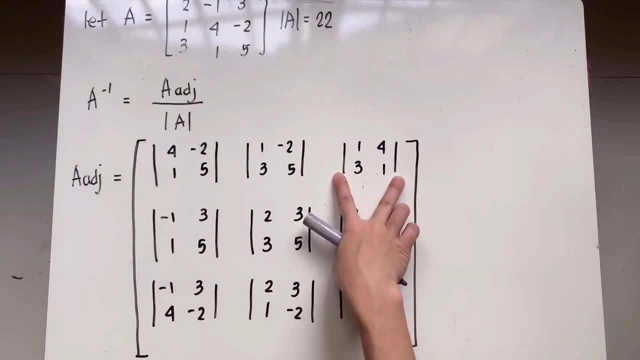 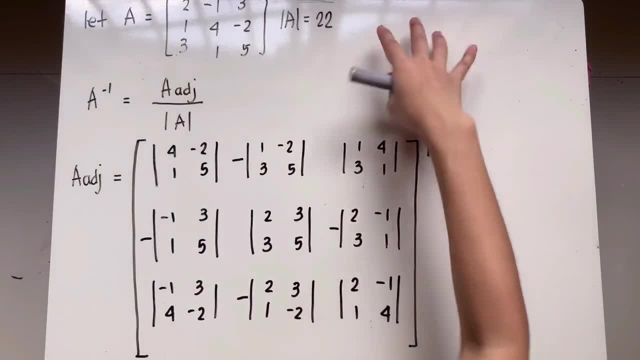 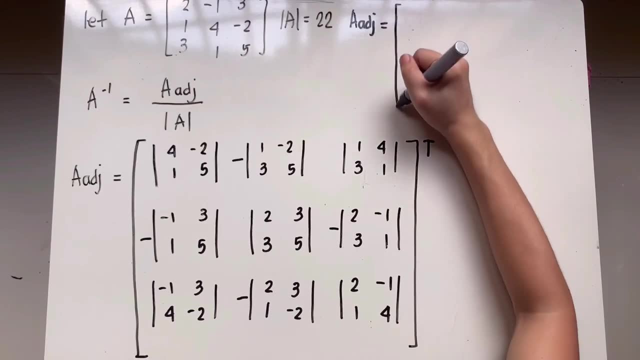 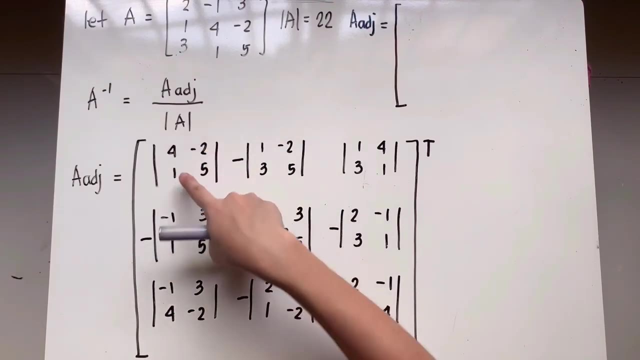 And that gives you your adjoint matrix. So let's continue that over here. I think it fits. So for A adjoint that would be equivalent to: So we have 20 minus 20 minus negative 2. So you get positive 22 for that. 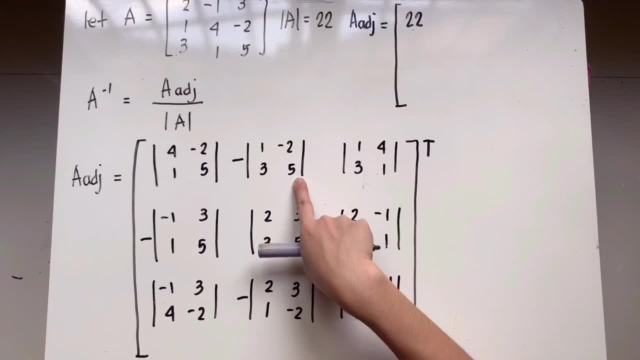 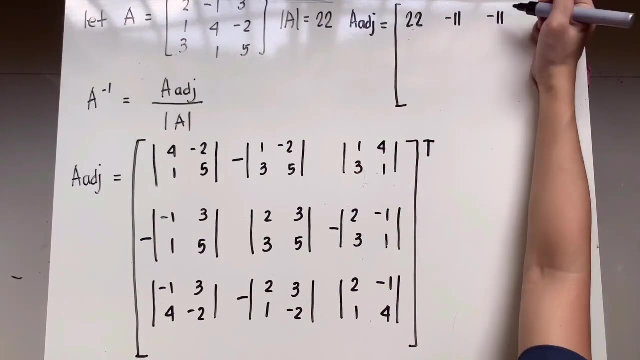 This one is 5 minus negative 6. So that's 5 minus negative 6. That's 11 times negative 1. So you get negative 11. You get 1 minus 12. So you get negative 11 again. 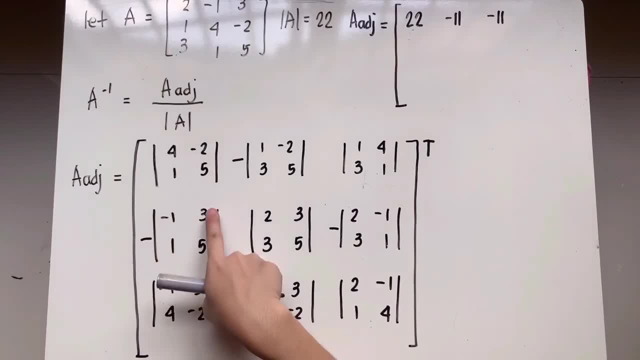 This one is negative, 5 minus 3. Negative: 5 minus 3 is negative, 8 times negative: 1. You get positive: 8. You get 10 minus 9. So you get positive: 1. You have 2.. 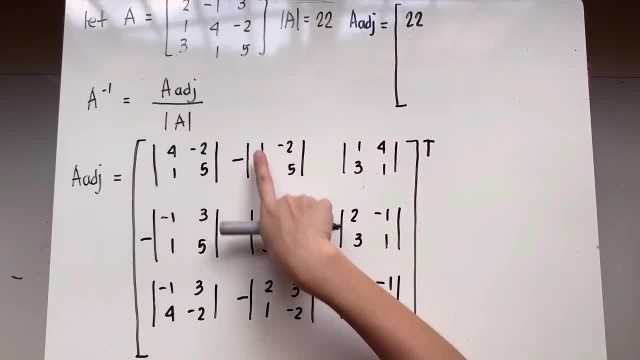 So you get positive 22 for that. This one is 5 minus negative 6. So that's 5 minus negative 6. That's 11 times negative 1. So you get negative 11. You get 1 minus 12.. 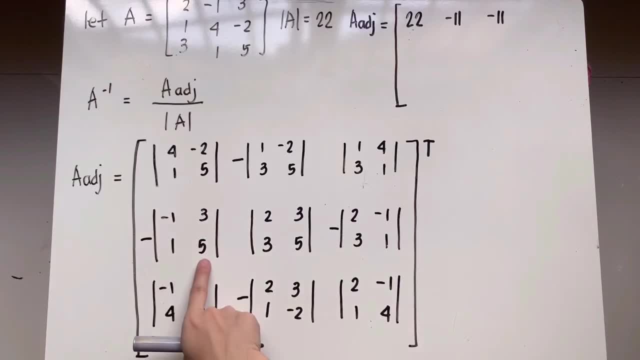 You get negative 11 again. This one is negative, 5 minus 3.. Negative 5 minus 3 is negative, 8 times negative 1. You get positive 8.. You get 10 minus 9. So you get positive 1.. 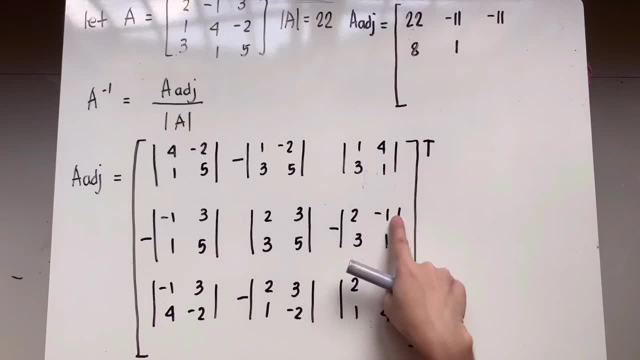 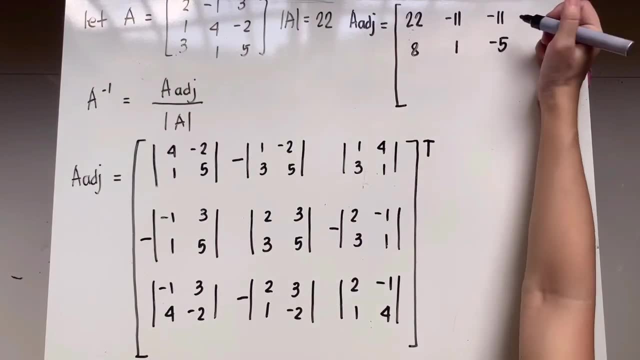 You have 2.. 2 minus 3. Sorry, 2 minus negative 3. So you get 5 times negative 1. So you get negative 5. We have positive 2 minus 12. So that's negative 10.. 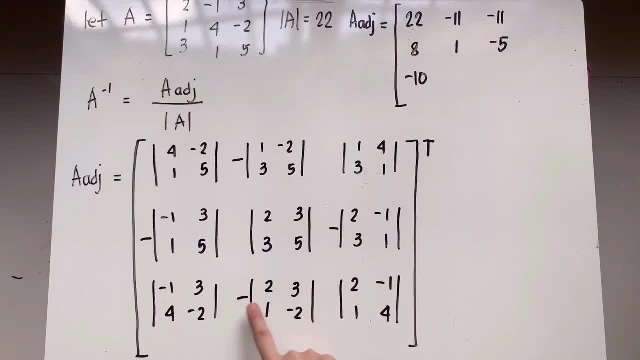 Negative 4 minus 3. So we get negative 7 times negative 1. That's positive 7. We get 8 minus negative 1. So we get positive 9. And then for that we transpose that matrix. 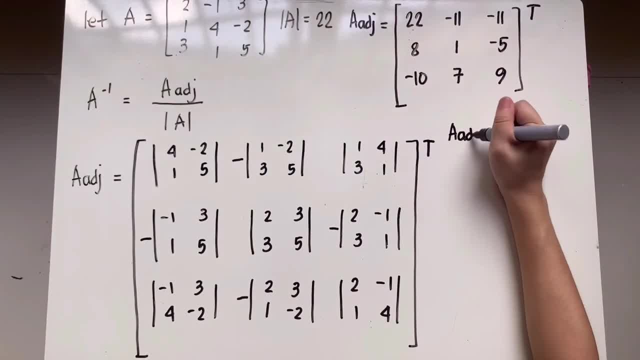 So your A adjoint is actually the transpose of this matrix, And that would be 22,, 8, negative, 10. Negative, 8. Negative 10. Negative 11,, 1, and 7. And negative 11, negative, 5,, 9.. 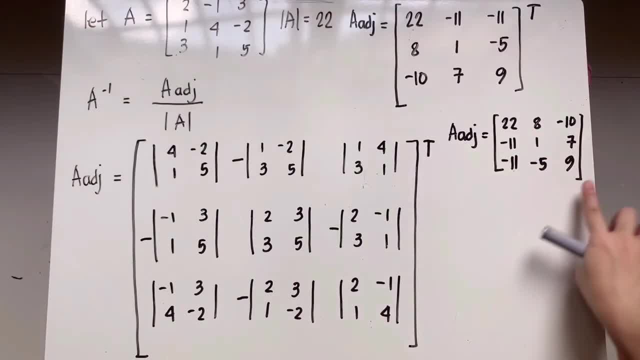 So I shifted the columns to rows. That's your A adjoint. Okay, Upon getting A adjoint, you have to divide it by the determinant. You are going to have your A inverse, So let's solve that On this side. 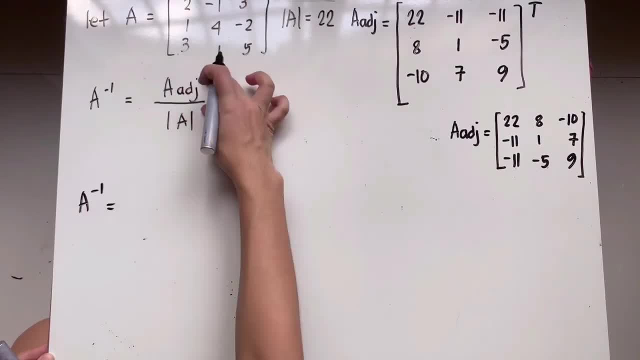 Our A inverse, therefore, is equivalent to your adjoint matrix, which is this one. So let's solve that. So let's copy that. That's 22,. negative 11, negative 11,, 8, 1, negative 5, negative 10,, 7, and 9.. 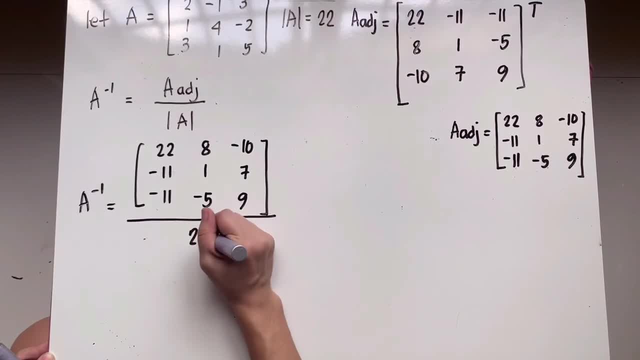 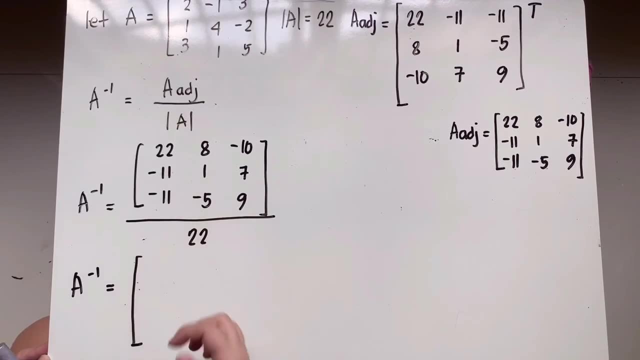 Divided by the determinant we had, which is 22.. So we'll be able to simplify our A inverse as So: 22 divide 22,, that's 1. Negative 11.. 11 divide 22 is negative 1 half. 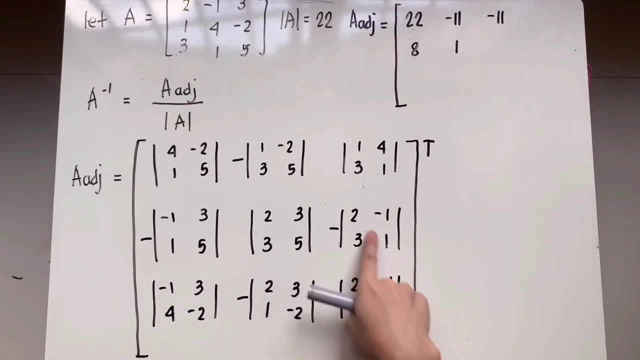 2 minus 3. Sorry, 2 minus negative 3. So you get 5 times negative 1. So you get negative 5. We have positive 2 minus 12. So that's negative 10. Negative: 4 minus 3.. 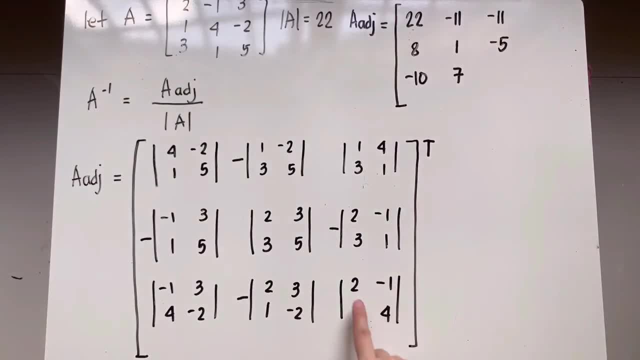 So we get negative 7 times negative 1. That's positive 7. We get 8 minus negative 1. So we get positive 9. And then for that we transpose that matrix. So your A adjoint is actually the transpose of this matrix. 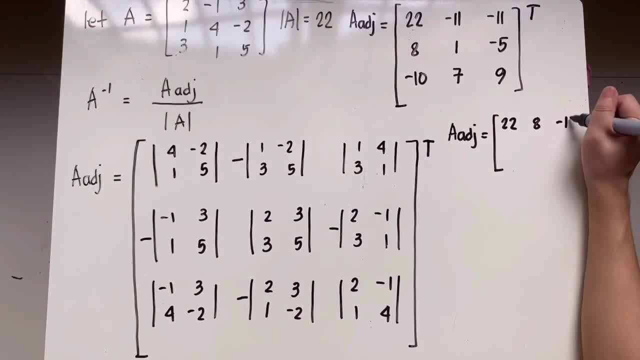 And that would be 22.. 22. 8, negative 10, negative 11, 1, and 7, and negative 11,. negative 5, 9.. So I shifted the columns to rows. That's your, A adjoint. 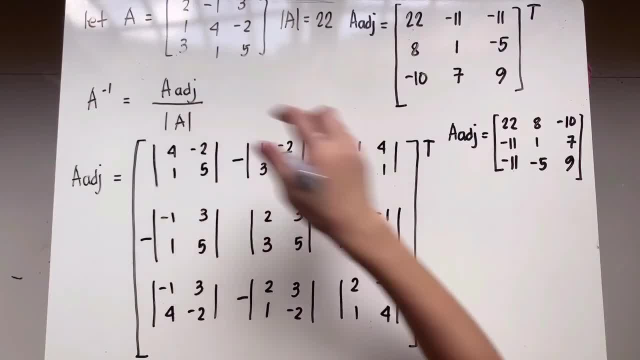 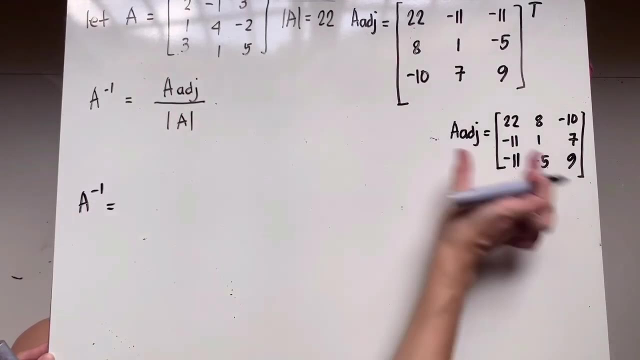 Okay, Upon getting A adjoint, you have to divide it by the determinant. You are going to have your A inverse, So let's solve that on this side. Our A inverse, therefore, is equivalent To your adjoint matrix, which is this one: 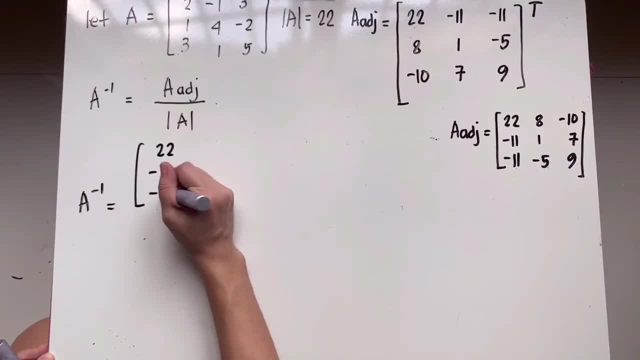 So let's copy that, That's 22,. negative 11, negative 11,, 8,, 1, negative 5, negative 10,, 7, and 9.. Divided by the determinant we had, which is 22.. 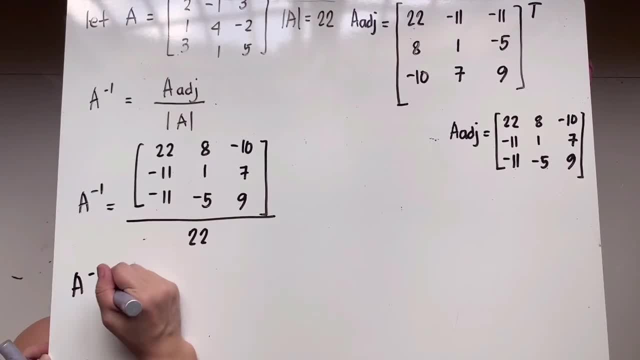 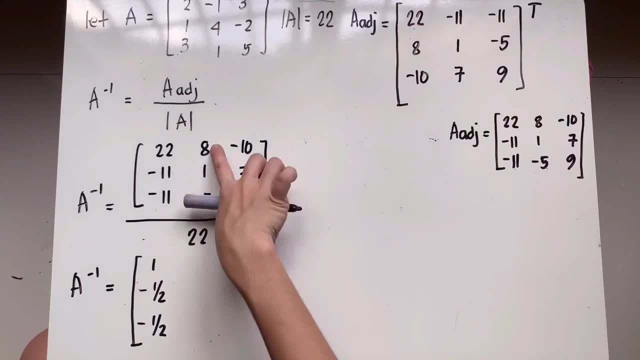 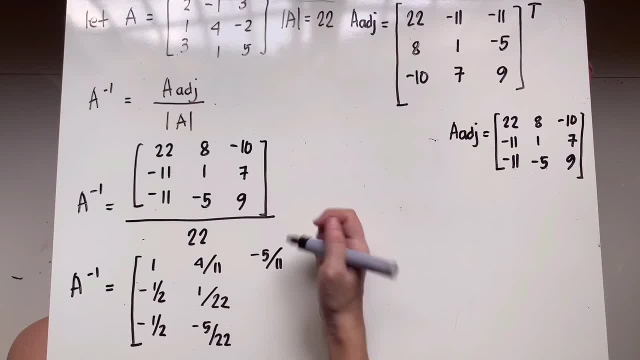 22. 22. 22. 22. 22. 22. over 22, and we have 9 over 22, that's 9 over 22. therefore, this is our a inverse. okay, recalling the solution we've had previously to solve for xyz. 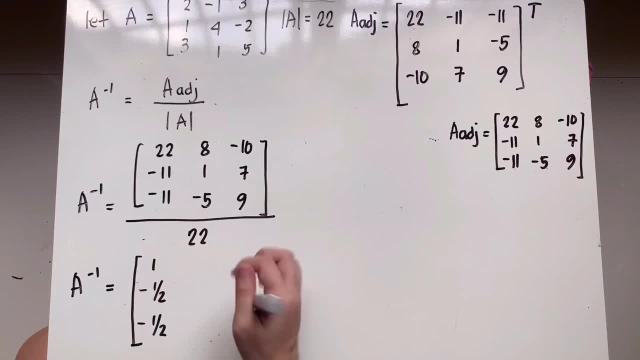 Negative: 11 divide 22 is negative 1 half. Next we get 8 over 22,, that's 4 over 11.. 1 divide 22,. that's 1 over 22.. Negative: 5 over 22,, that's negative 5 over 22.. 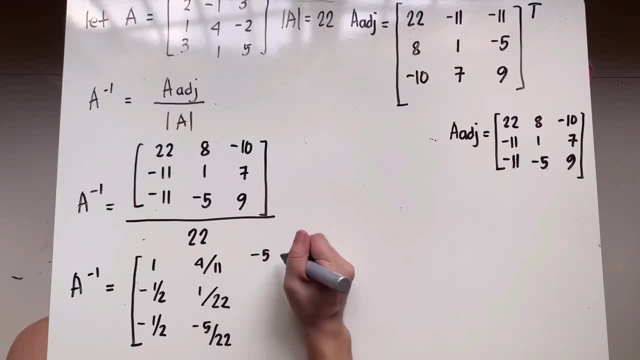 Negative 10 over 22,. that's negative 5 over 11.. We have 7 divide 22,. that's 7 over 22.. And we have 9 over 22,. that's 9 over 22.. therefore, this is our a inverse okay, recalling the solution we've had previously to solve for xyz. 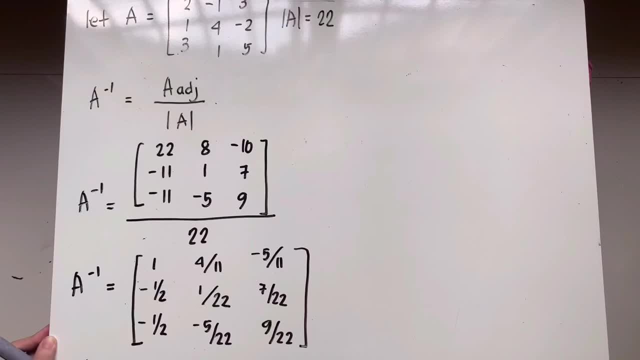 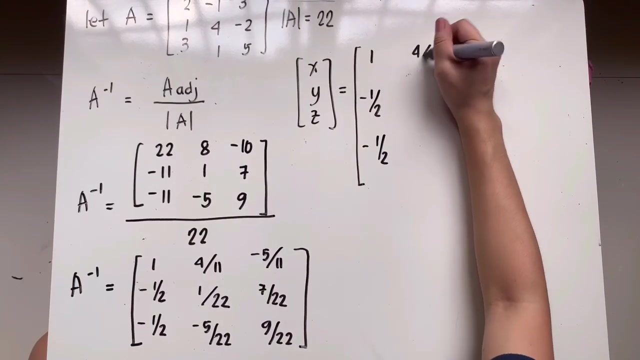 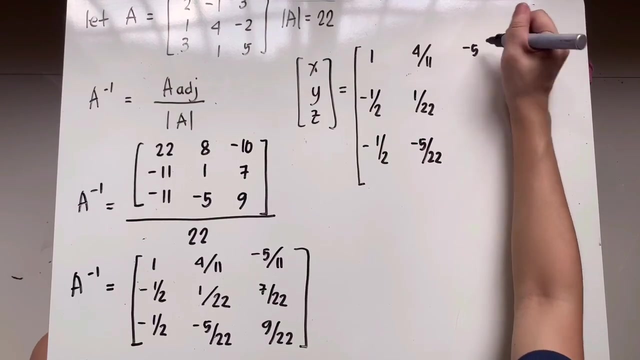 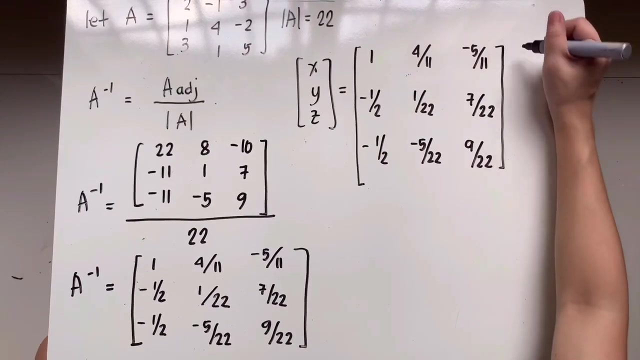 your xyz is equal to the product of a inverse. okay, that is 1 negative, 1 half negative, 1 half, 4 over 11, 1 over 22 negative, 5 over 22 negative, 5 over 11, 7 over 22 and 9 over 22. that would be multiplied to our constant. 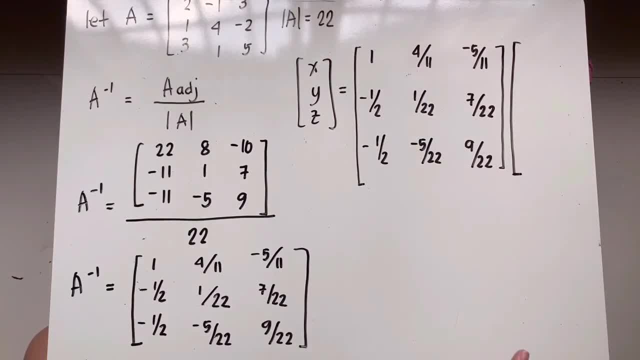 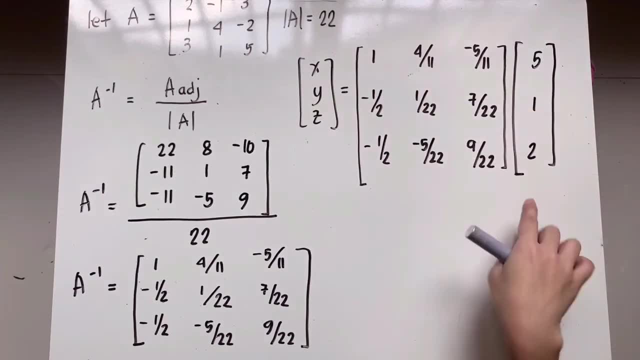 matrix, you may matrix of constants that we have, and that is 5,, 1, and 2.. After that we'll proceed with multiplication, right? So to solve for x, y, z, we are going to take the product of this. 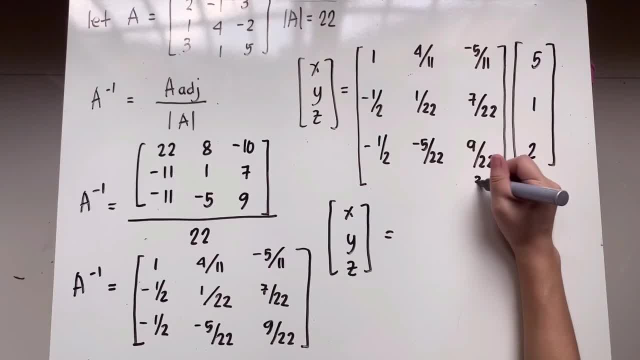 This is 3 by 3 times 3 by 1.. So 3 by 3 multiplied to 3 by 1, you'll get a 3 by 1 answer, which means we'll get a single column vector as our answer And we'll proceed with multiplication. 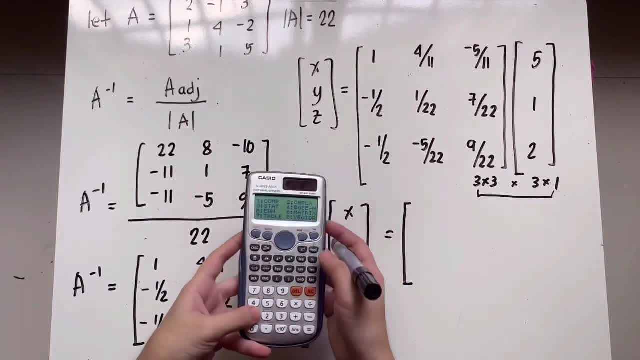 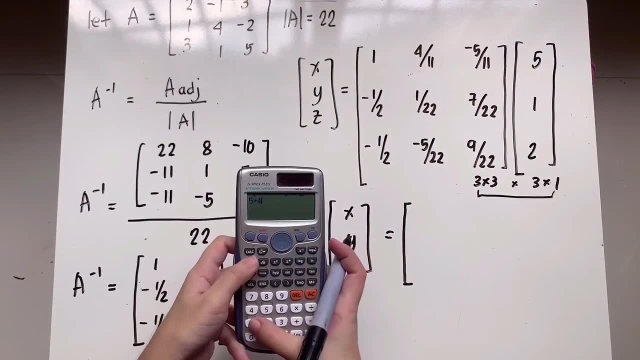 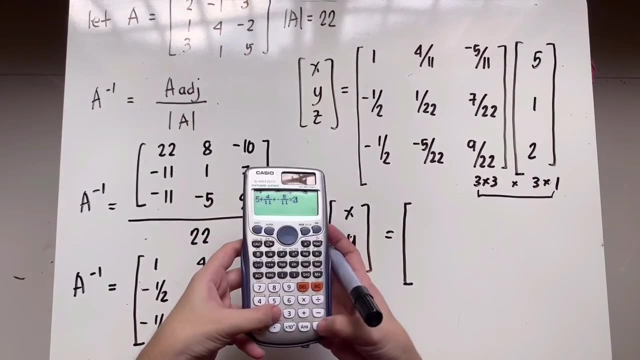 So let me get my calculator for that. So for our multiplication that would be 1 times 5 plus 4 over 11 times 1, that's 4 over 11, plus negative 5 over 11 times 2.. So negative 5 over 11 times 2.. 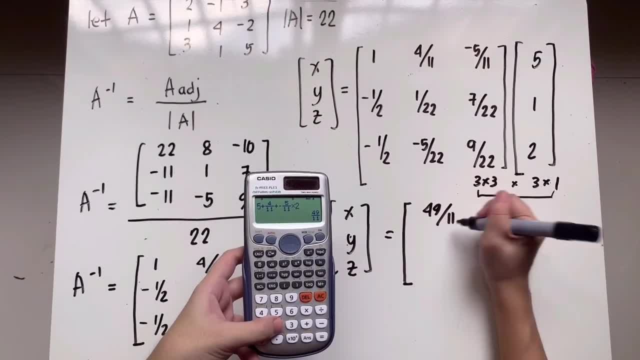 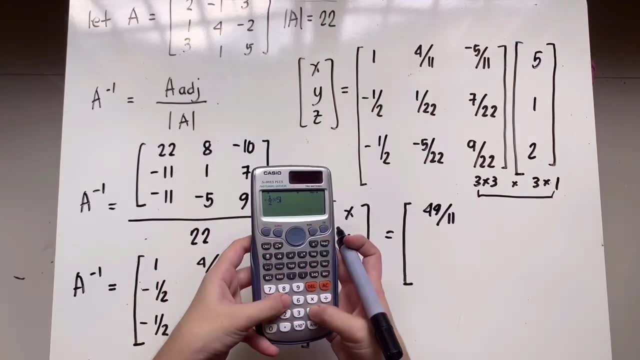 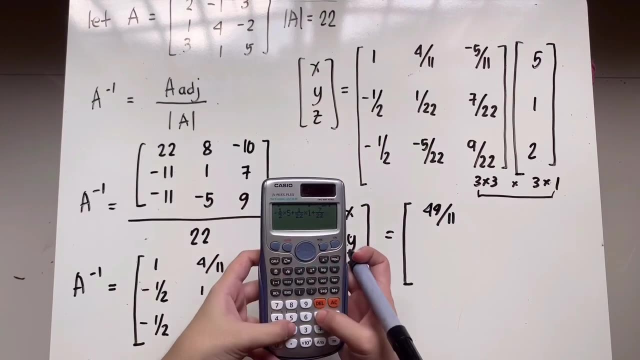 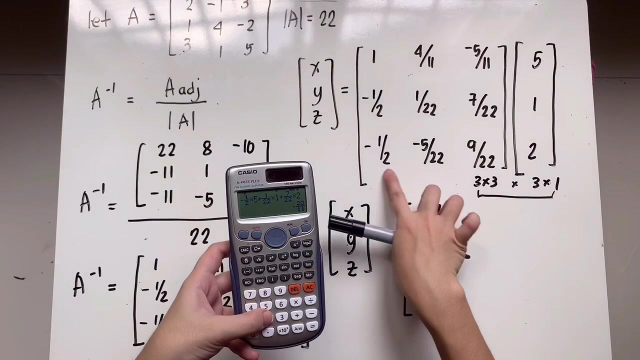 And that gives us 49 over 11.. Next, this row to this column naman. So you get negative 1 half times 5 plus 1 over 22 times 1 plus 7 over 22 times 2. And that gives you negative 20 over 11.. Lastly, we go over the third row. 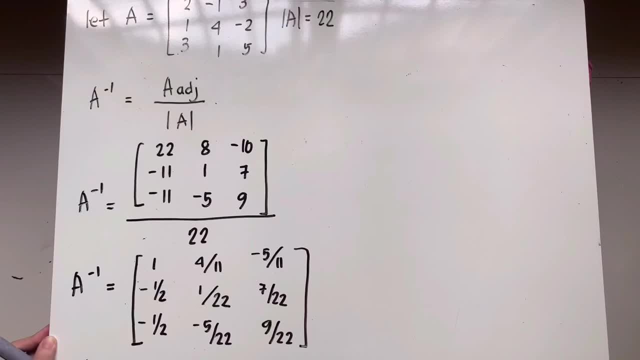 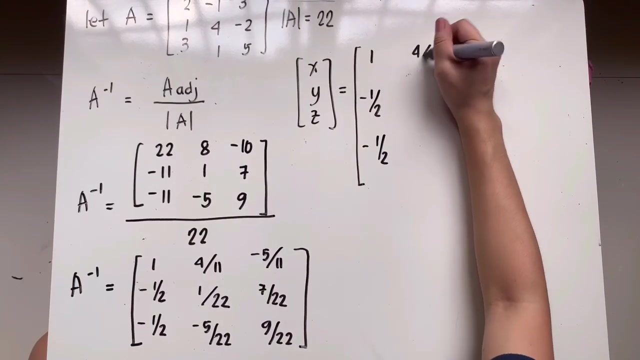 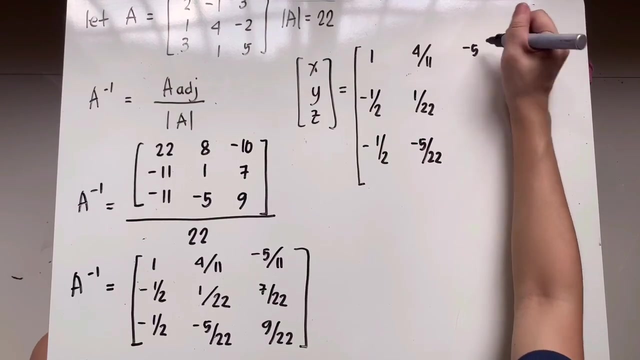 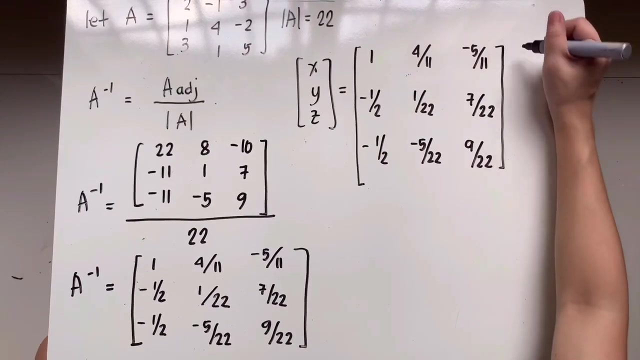 your xyz is equal to the product of a inverse. okay, that is 1 negative, 1 half negative, 1 half, 4 over 11, 1 over 22 negative, 5 over 22 negative, 5 over 11, 7 over 22 and 9 over 22. that would be multiplied to our constant. 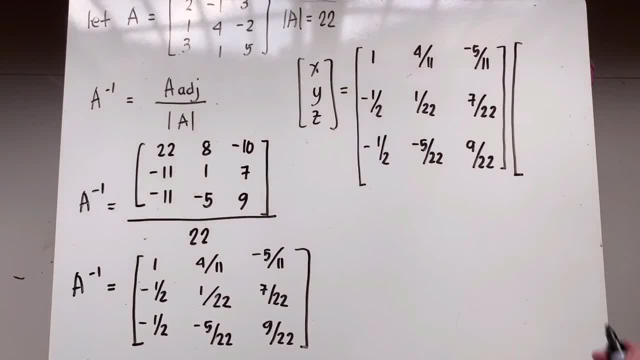 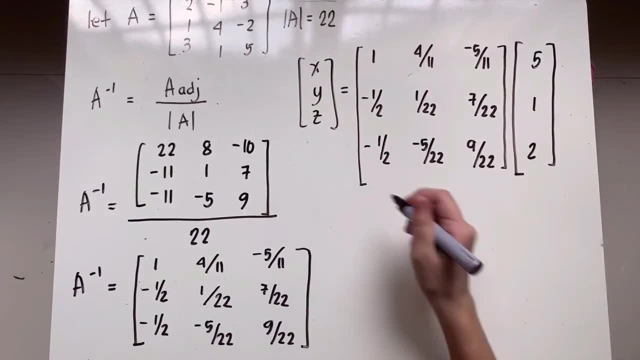 matrix, your matrix of constants that we have, and that is 5, 1, 12 and two. after that we'll proceed with multiplication, right? so to solve for x, y, z, we are going to take the product of this. this is three by three times three by one. 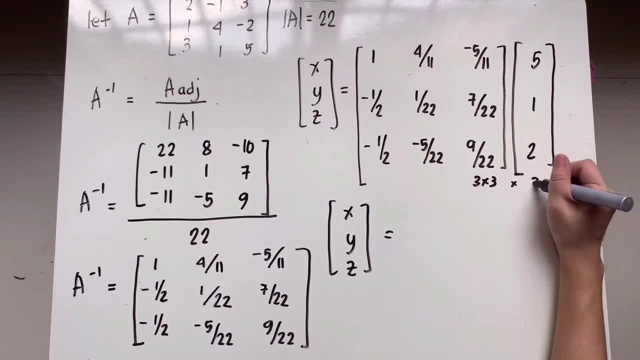 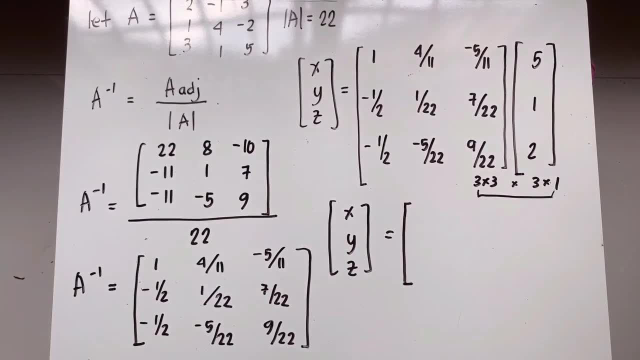 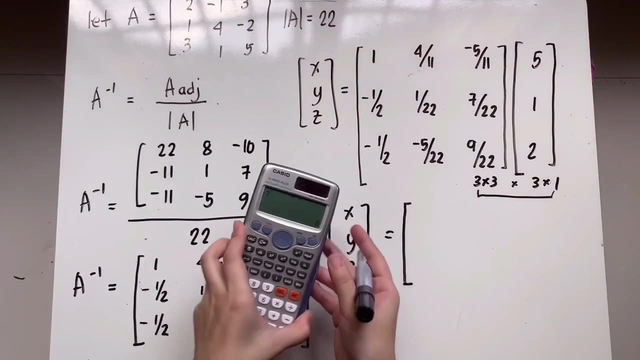 so three by three multiplied to three by one, you'll get a three by one answer, which means we'll get a single column vector as an hour, as our answer, and we'll proceed with multiplication on. so let me get my calculator for that. so for our multiplication that would be one times five. 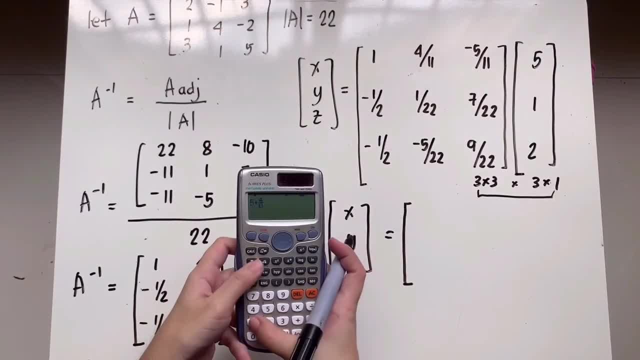 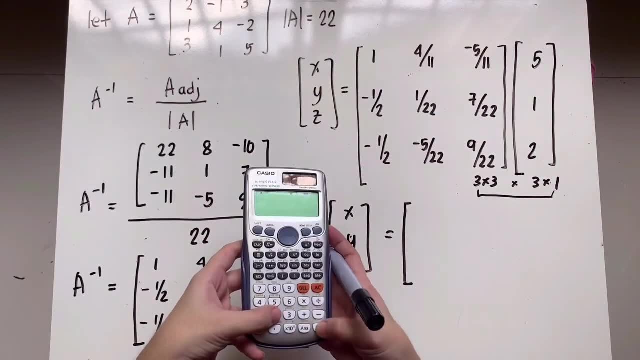 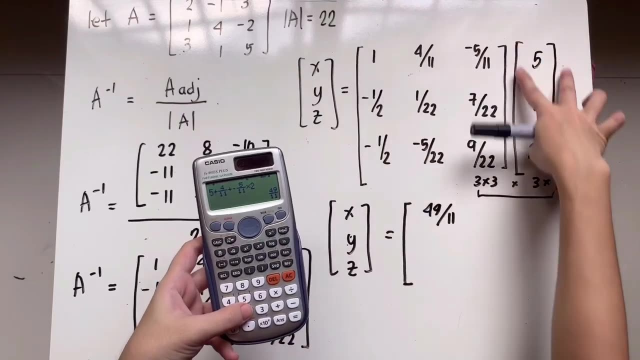 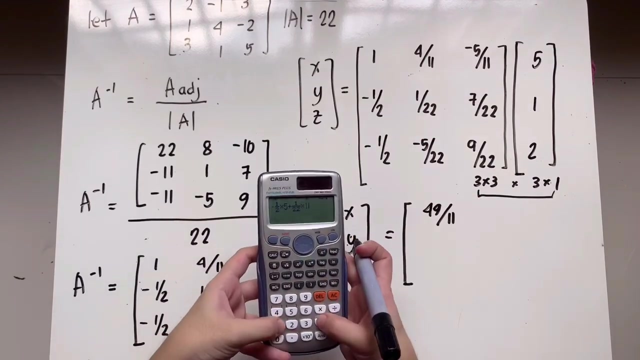 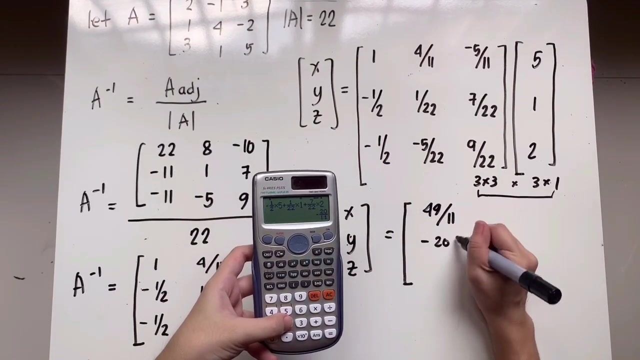 plus four over eleven times one, that's four over eleven plus negative five over eleven times two, so negative five over eleven times two and that gives us 49 over eleven. next this row to this, so you get negative one half times 5 plus 1 over 22 times 1, plus 7 over 22 times 2, and that gives you negative 20 over 11. lastly, 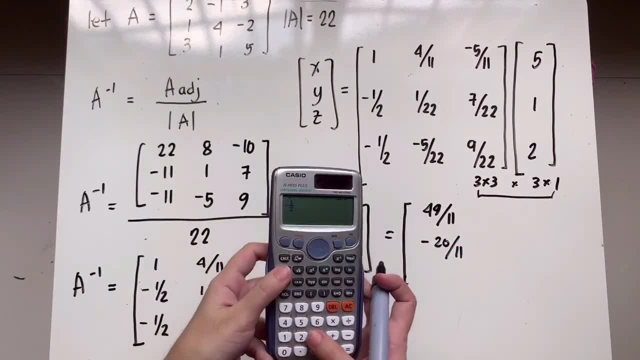 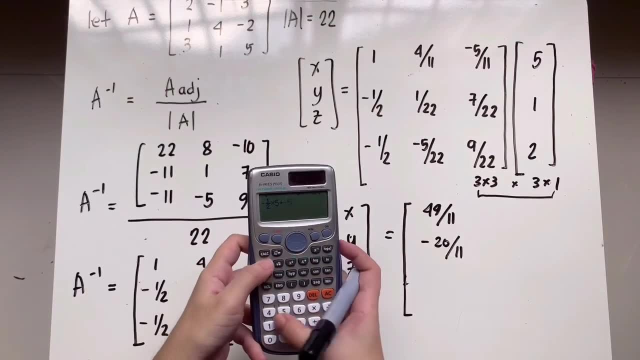 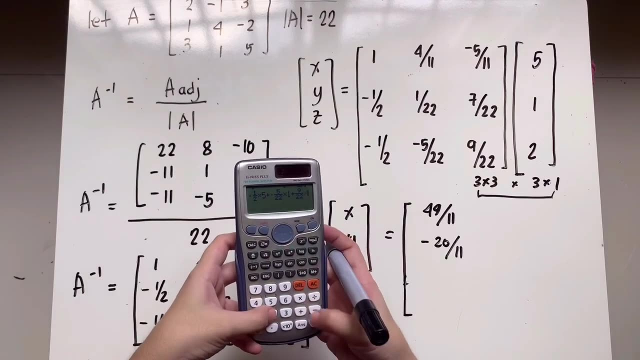 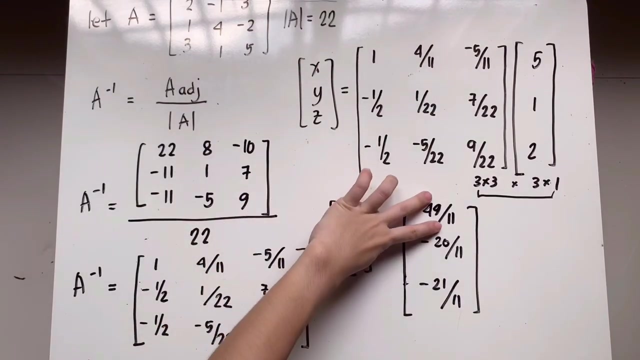 we go over the third row, that's negative one half times five again, plus negative 5 over 22 multiplied by 1, plus 9 over 22 multiplied by 2, and that gives us negative 21 over 11 and, if you've noticed, this means x is equivalent to this. 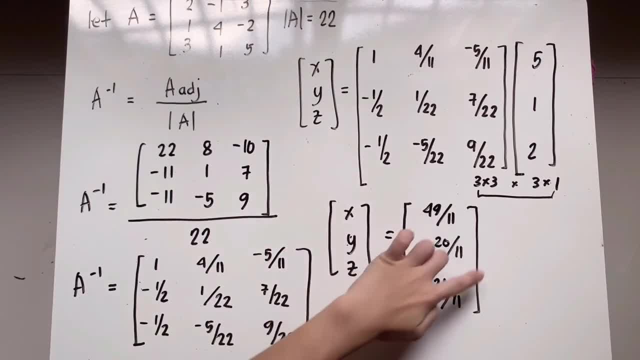 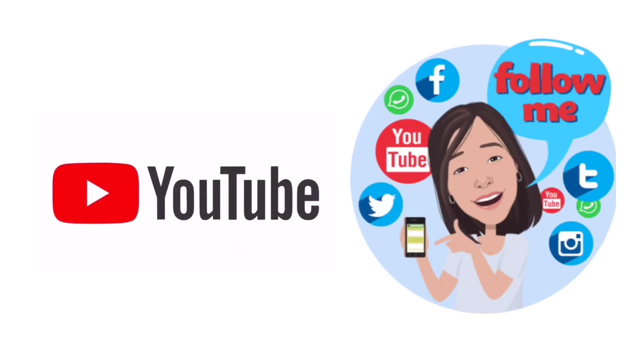 y is equivalent to this and z is equivalent to this, and all of these answers are the same answers we've had when we solved it using kramer's rule. so